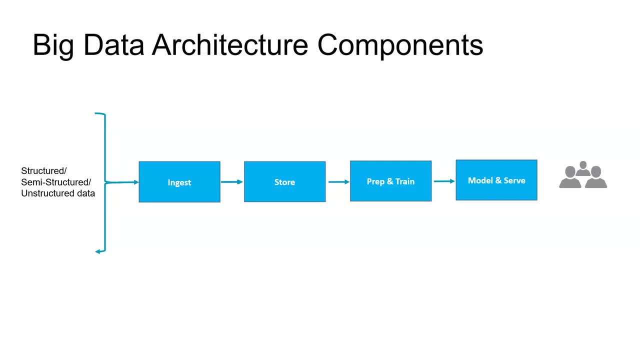 is called data ingestion. Data ingestion tools help to collect, import, load, transfer, integrate and process the data from wide variety range of data sources. So it will just collect the data, whether you have a SQL Server, Oracle or MongoDB or some other. 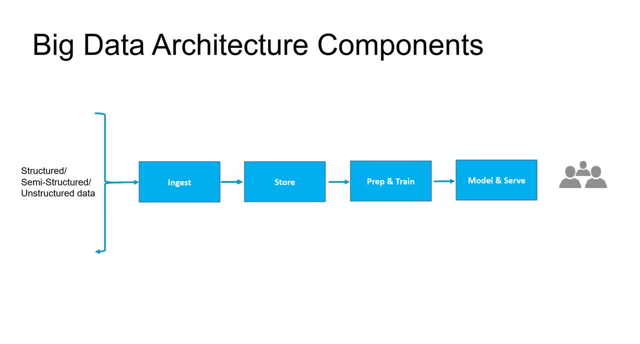 XYZ database or you have completely unstructured data. That will provide those tools, will provide some plugins to collect the data from the various sources. So the next step is store. So your store is considered an 찾ięcy tables where you can store the data, etc. As I mentioned there already. 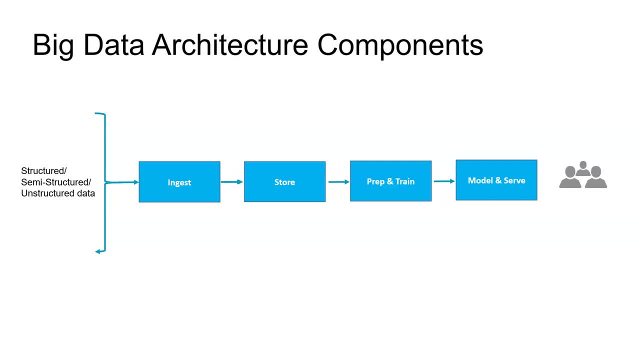 are certain ICünding tools. you have to go through and do some scouting and checking if you see there is an ICünding software that's startled the content that the science was instituting. So if you have the ICünding software you can try. etch it on your name and this method. 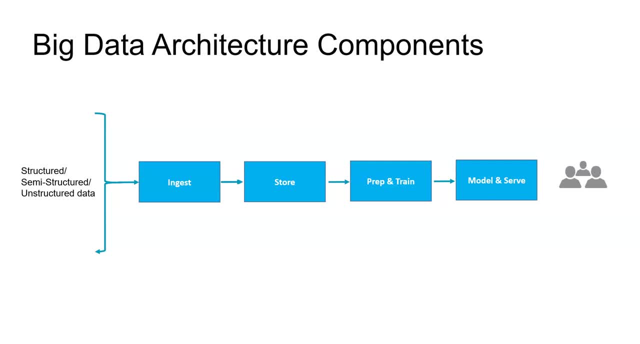 is better SUV, okay. So without telling anyone that you would describe of a possible CC Kr♥d overseas website, you will want to use it. That should not be visible on your site, right, but not from the dirt nosotroscom. So complete log. 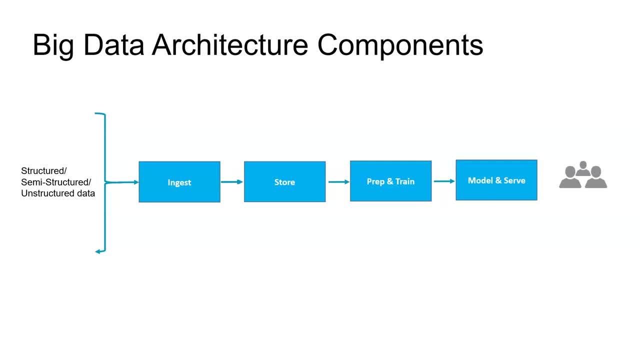 never know like what it comes. we can't predict what kind of data comes from there, right? so this story should be capable to handle that, whatever the data coming through the ingest, and to store the data in the stories. the third step is prep and train. so during the preparation and training, the data need. 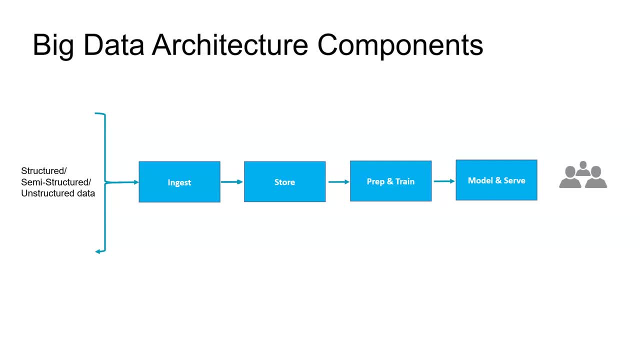 to be prepared. first because the variety of data is stored in under the stories so that data sets need to be taken and that need to be trained to generate the machine learning models. that means, like you want to create a predictive analysis based on the previous months of data, you can prepare the data and then you can. 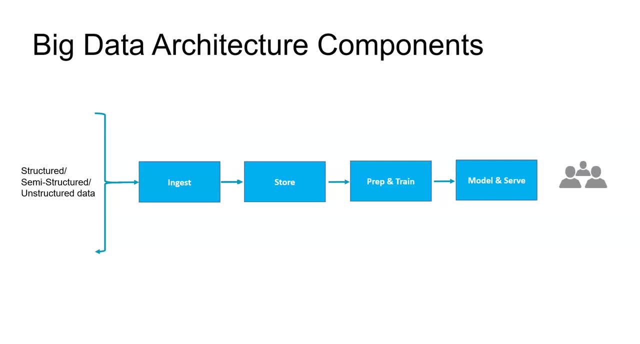 train the data as per your requirement. so there are two major parts in this. one is preparing the data: first, collecting the data from the stories and preparing the data. then you need to train the models as per your requirement, whether it could be just performing simple analytics like seeing the what happened. 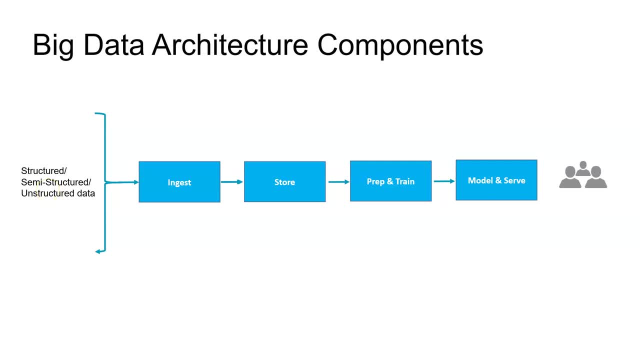 in the previous months, or you can predict for the next few months sales or how the resources usage is going to be. all those stuff can be prepared by using this. the next one is model and so, so this can also be called as data warehouse. the data could be used as a model, and so this can also be called as data warehouse. so this can also be called as data warehouse. the data could be. 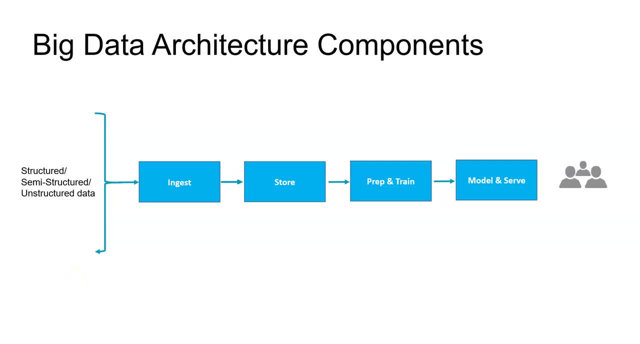 in the form of predictions based on the machine learning models which are prepared in prep and train, are in a structured form for analytical reporting based on the business intelligence use cases. so all this data will be stored in data warehouse. that means the analyzed data or the training based output will 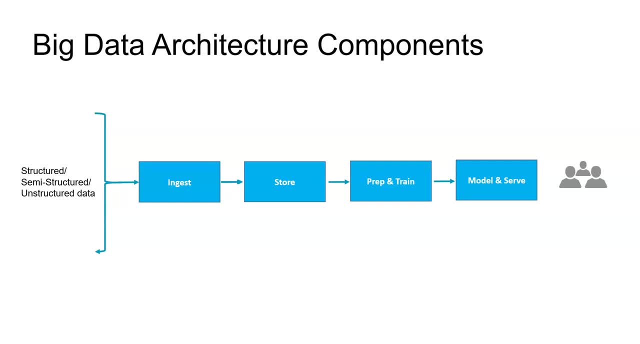 be stored in the data warehouse from here that need to be served to the UI. that means the end user need to see in the form of the dashboards or some beautiful you, a format, so this model and serve will serve the data to build. the custom reports are the. 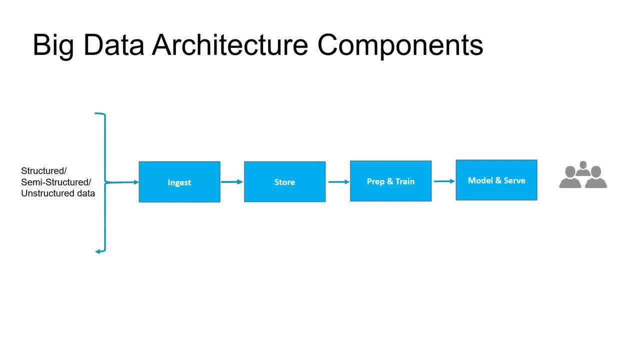 beautiful reports so that the end user can see those reports and they can take their calls as per for their sales or for their next projections and stuff. so any big data architecture should be constructed based on this four building blocks or four components. so let us see what tools we can use for injections, store, prep and train and model and serve. 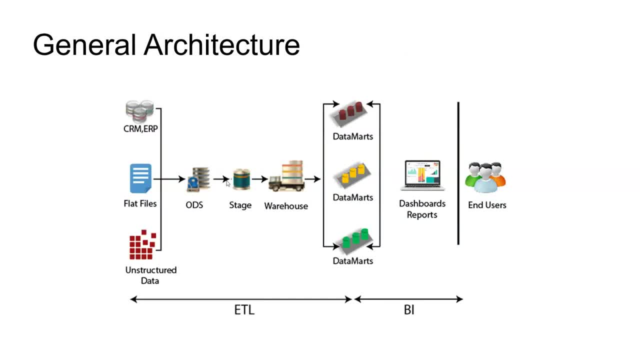 so let us go for next one. so this is the earlier of our architecture, like 10 years ago, if you see how the this type of actions or components were being performed. for example, there are different types of data coming from various resources, various sources like crmerp, flat files and 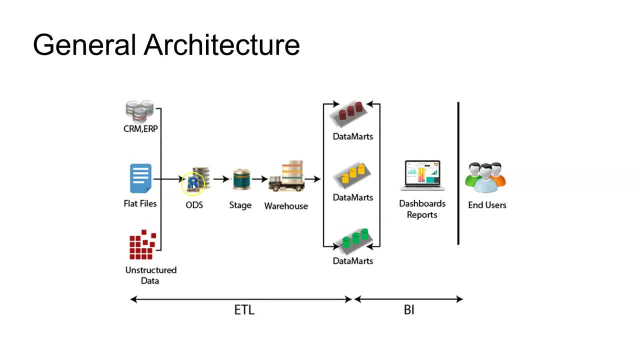 structured data is coming to the ods which is being ingested like the data is ingested through the ods, and it will be staged somewhere that is a storage and then there will be a data warehouse where it will be like model and serve. then it will be sent to the data dashboard reports. 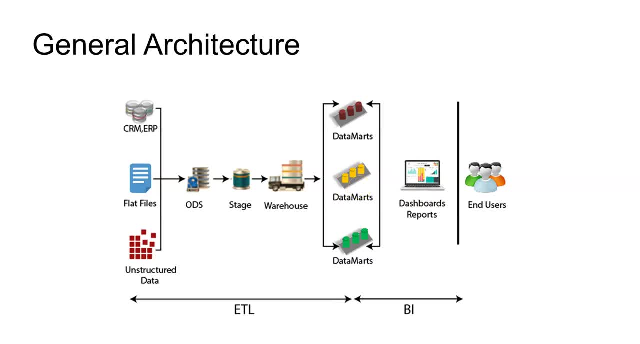 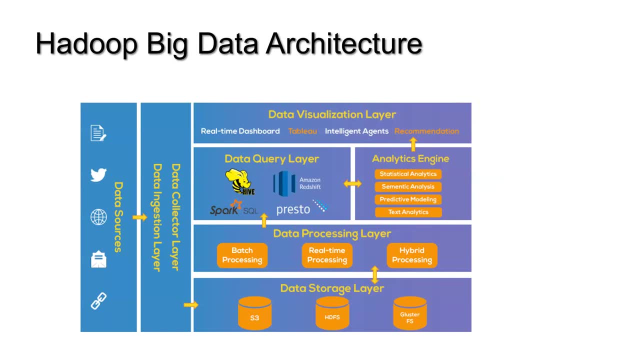 so this is how the big data architecture was performed, like 10, 15 years ago now. the next one is: how do big data architecture so nowadays, when you call it big data, immediately they say: how do? or you talk about big data analytics, they immediately respond with the term of hudu. not every big data is hudu there. 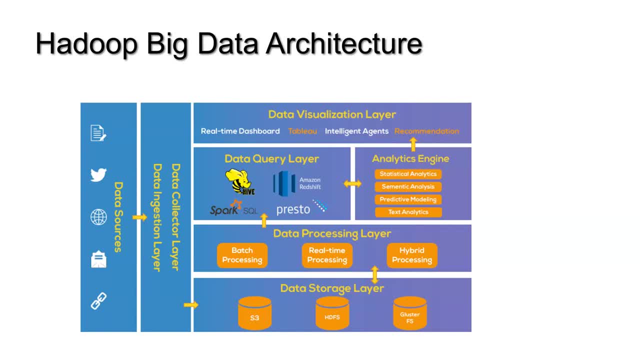 are plenty of tools available. you have to select which is best for your requirement. so you you have to aware like: what are the things available? azure provides, how do provides, aws provides, gcp provides plenty of options. you need to actually analyze what is best for you. what are the pros and cons of each? 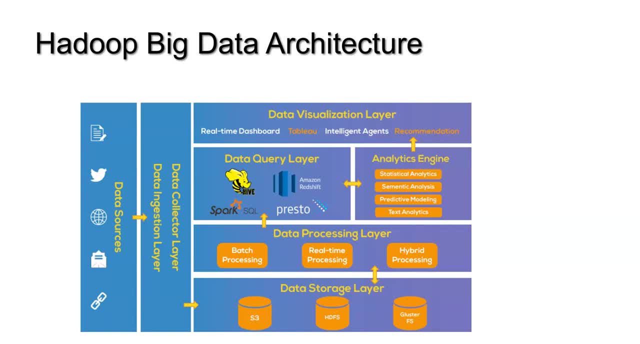 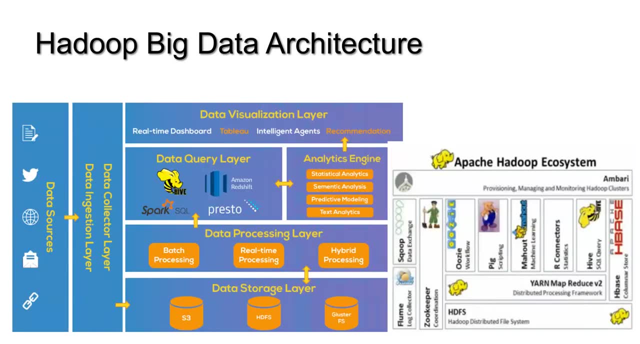 and every component, and then you need to come to the conclusion which will be the best one for you. so how do? is just not whole and soul for the big data architecture? there are plenty of options available. so apache, hadoop system- you can see here. there are data ingestion tools like scoop. 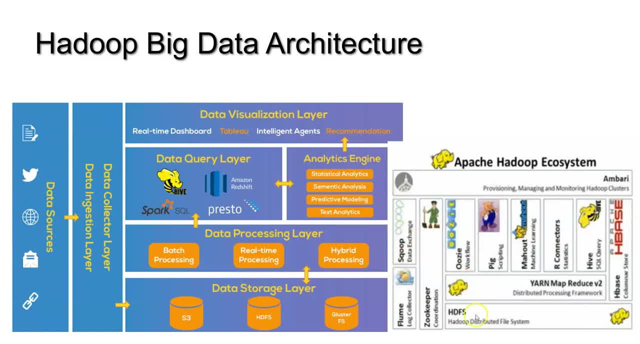 these are the data ingestion tools and for the stories they have used hdfs, hadoop, distributed file system. and then you have a h base for the real time processing. for the generic data processing you have spark, map, reduce, hive and all those stuff you can see here for real time processing. 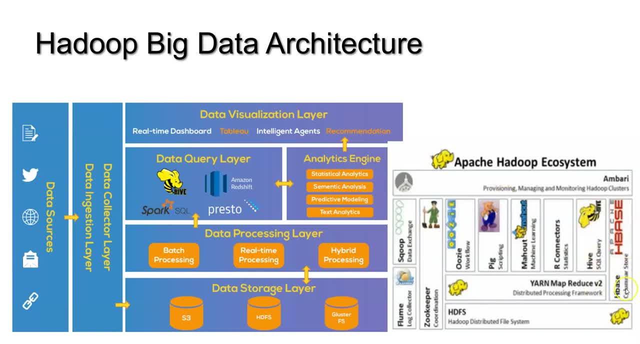 you have h base. you can see at the corner h base. so for ba and visualization, you can see hive here. so that's how you know. every architecture will have those four components for the ingestion, store, prep and train and then model and serve. so, however, in the hudu system also you can see all those components but you have to explore variety of. 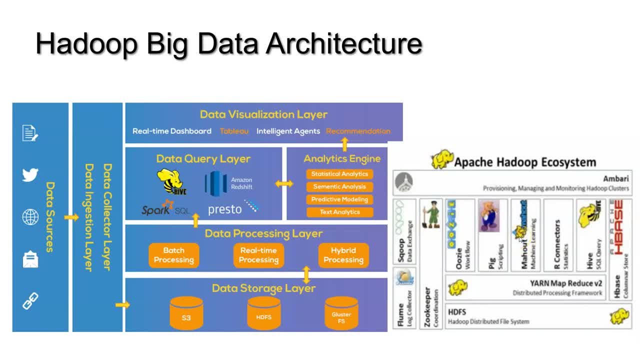 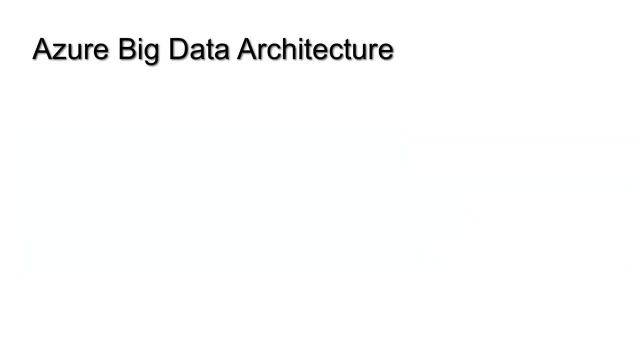 components which can match for your requirement. let us jump into our main agenda of this presentation, that is, azure data architecture. so here it is azure big data architecture. as i mentioned, there are plenty of sources which generates the data and the data need to be read from those data sources by using the data ingestion. 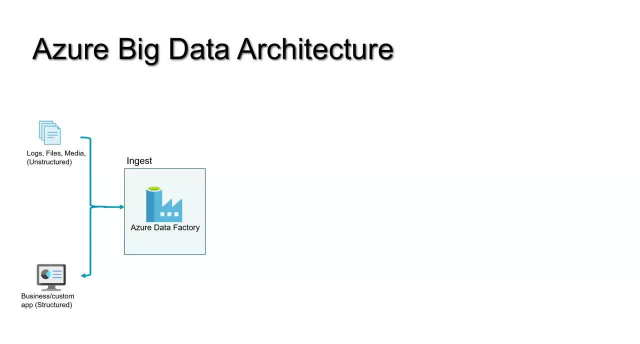 tool. so the suitable data ingestion tool on the azure is azure data factory. so azure data factory will help you to plug into that particular data sources and to bring the data into the azure data storage. so azure data lake storage will help you to store plenty of the data, like it could be. 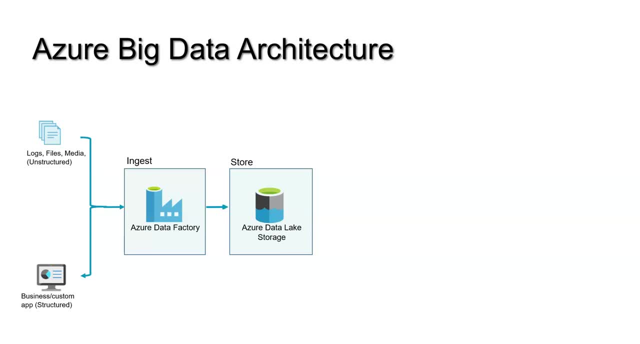 terabytes, uh petabytes or hexabytes of data into the storage. so azure data lake store is a gen 1 and azure data lake storage gen 2 are available. under azure data lake storage gen 2 you can select blob stories, which is a general storage. with that you can get many advantages, like lrs, zrs, grs. 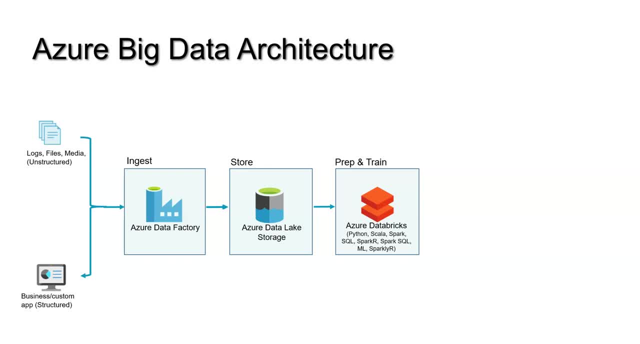 and other advantages to store the data. so, coming to the azure databricks, azure databricks help you to curate and process massive of data and developing, training and deploying models on the data, and also to manage the whole workflow process. assume that you have a plenty of data on the data. 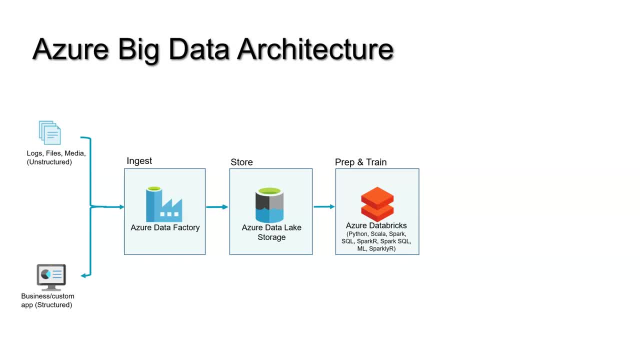 lake storage like hexabytes of amount of data. now you want to write some predictive analysis, or you want to just see what was a sales in past one year and based on that, you want to take certain decisions, like your csu team or your senior management team wants to take some. 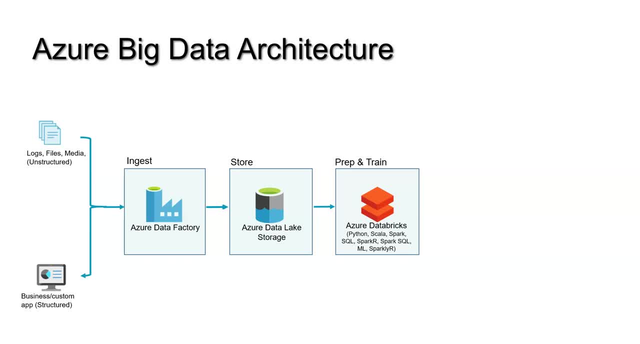 decisions. so first you need to train your models so that it can help you to bring the data in: how that sale is going to be in next few months, or how the resource utilization going to be in next few months or next year, so all those predictive analysis can be written. 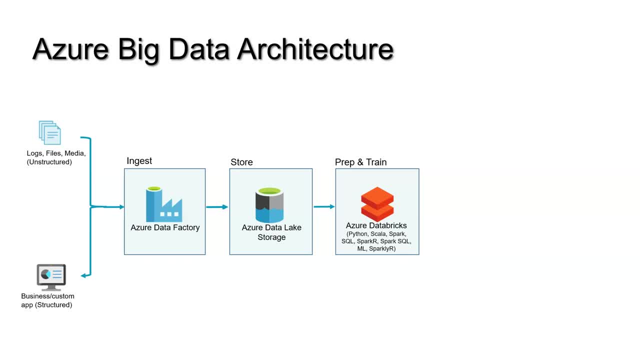 by using your machine learning concept. that is like python, scala. all these programming languages will help you to write, so such kind of models. so, in case, if you think that azure databricks, uh, is not only the option, then you can also use azure hd, insight or polybase. 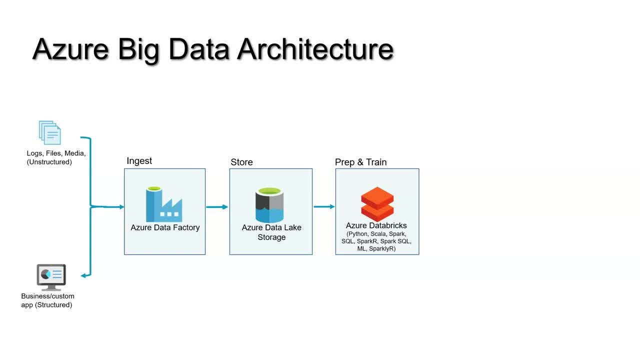 or azure data analytics. so all this will help you to write uh or do preparation and training on your data available on the storage. the next step is data warehouse. so here azure synapse analytics is considered as modern data warehouse. earlier you could see sql, azure sql data warehouse, but now 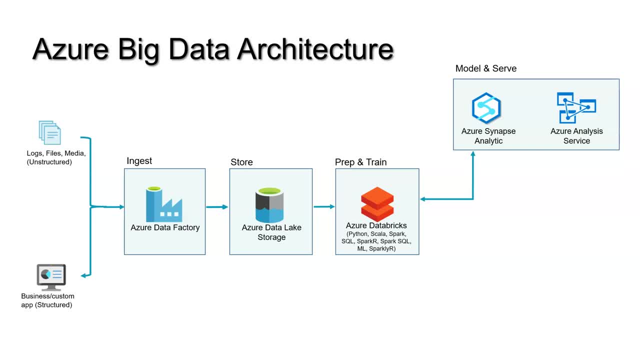 microsoft brought azure synapse analytics during last november releases, so azure synapse analytics is a limitless analytic service that brings together data warehousing and big data analytics, so it has the capability to process hexabytes of the amount of data and that's why they call they. 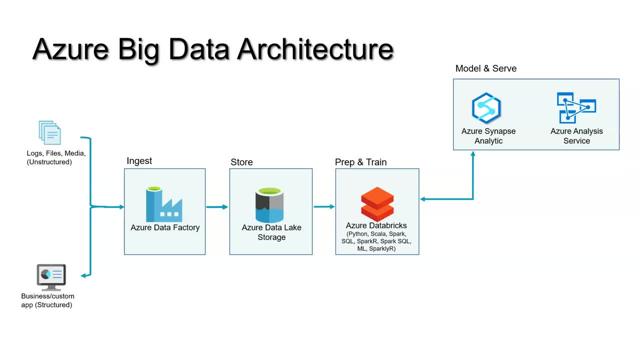 call it, or they claim it as limitless analytic service, so they can process the data to query and bring what you, what you required, and the performance is really good. it can even execute very complex queries within seconds. so microsoft claims that it takes a few minutes, whereas the big big query of the gcp takes a few minutes, or for the same query. 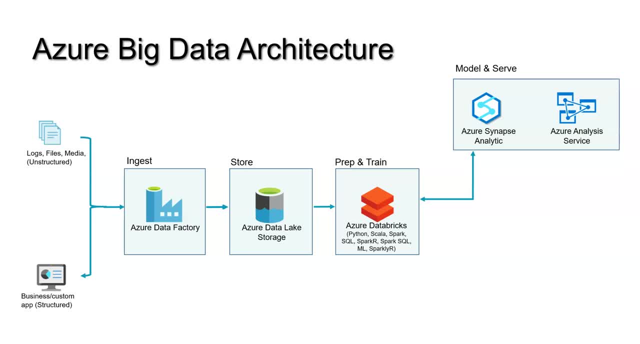 so that's how the performance of the synapse analytics. so you can also use an azure analysis service or azure sql data warehouse for the same place, like uh model and so so, as i mentioned, polybase also can be used to connect uh to the store and perform the synapse analytics on that. 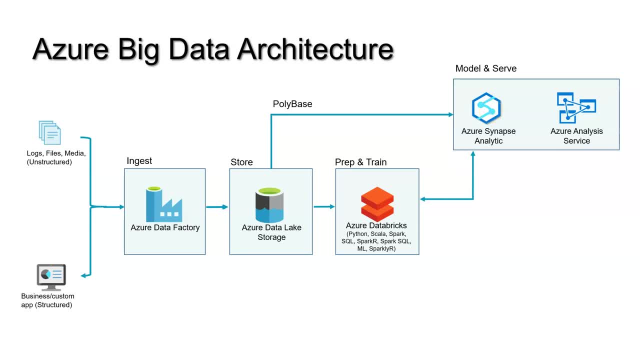 now you got the data and, uh, you can use the synapse analytics on that. now you got the data, you could perform some analytics on that. you know you need to project that to the ui because your senior management team should understand in the beautiful dashboards or some kind of beautiful ui format, right, so for that you can use power ba or there. 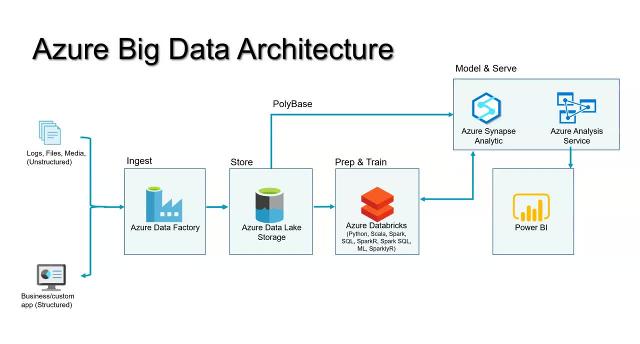 are plenty of other tools. like you can just simply connect to this uh as you synapse analytics and bring the data to that particular ui. so here i mentioned microsoft power bi. power bi is not some new tool, which is something new. it's safe from so many years. it will help you to plug in into the. 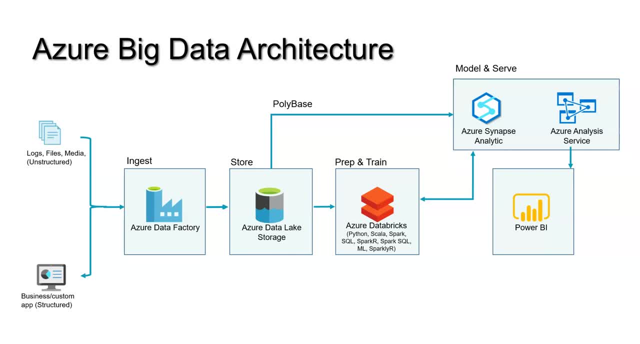 multiple data sources or there are 200 plus plugins on the power bi so you can plug in into the data source and then you can bring that and display it on the beautiful charts and different ua formats. so that's how the big data architecture works on the azure, but we can also see what are the alternate. 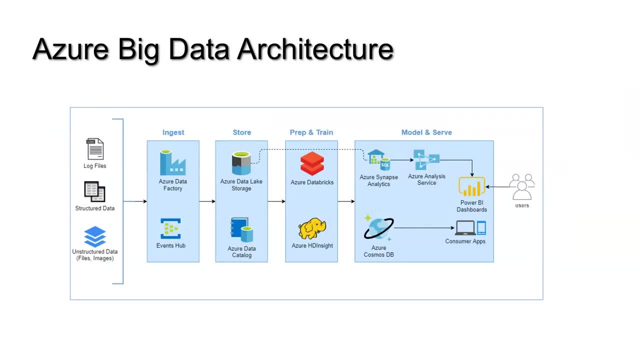 options available on the azure. let us go to the next slide. So, as I mentioned, every data architecture, big data architecture- got Ingest Store, Prep and Train Model and Server. But you can also use Events Hub. You can use Azure Data Catalog, Azure HD site for the Prep and Train.